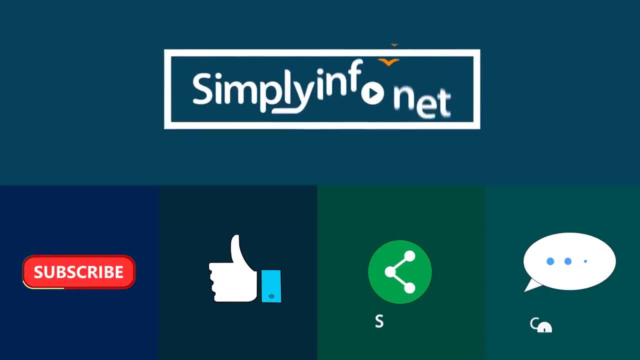 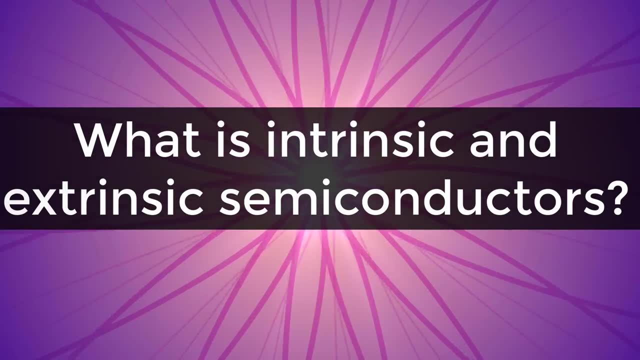 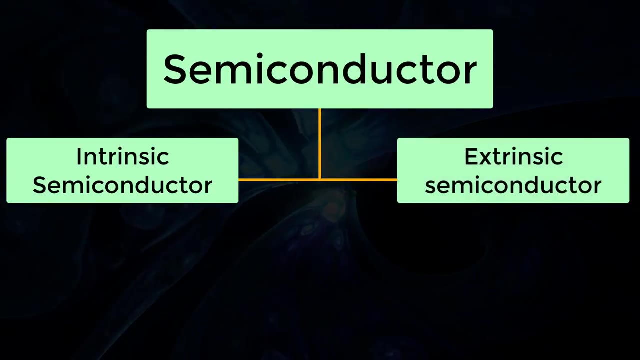 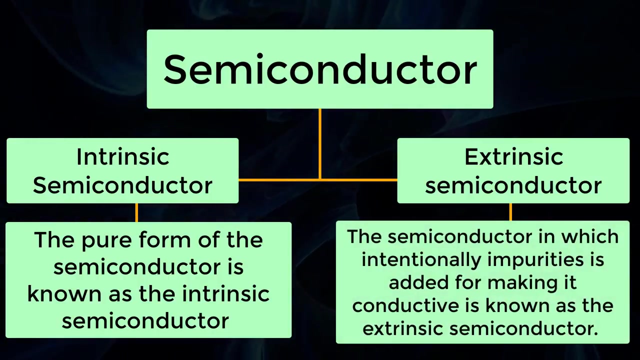 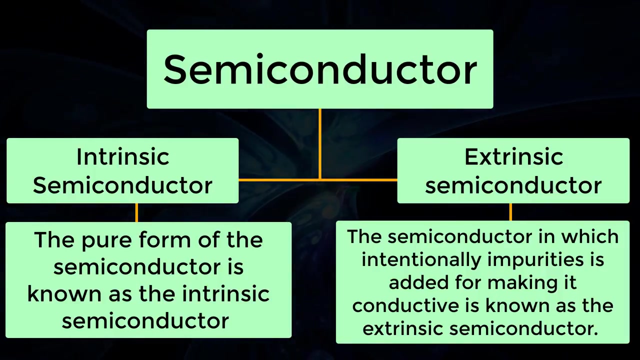 What is Intrinsic and Extrinsic Semiconductors? The semiconductor is divided into two types: Intrinsic Semiconductor and Extrinsic Semiconductor. The pure form of the semiconductor is known as the intrinsic semiconductor, and the semiconductor in which intentionally impurities are added to make it conductive is known as the extrinsic 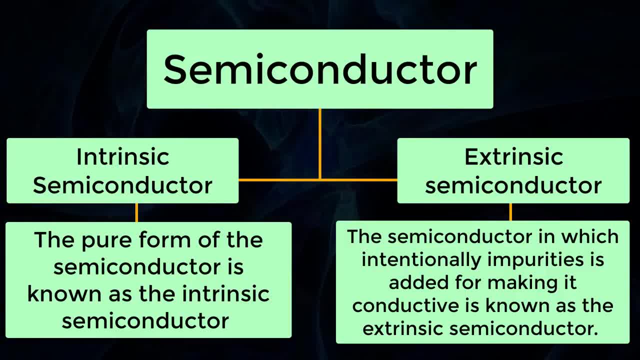 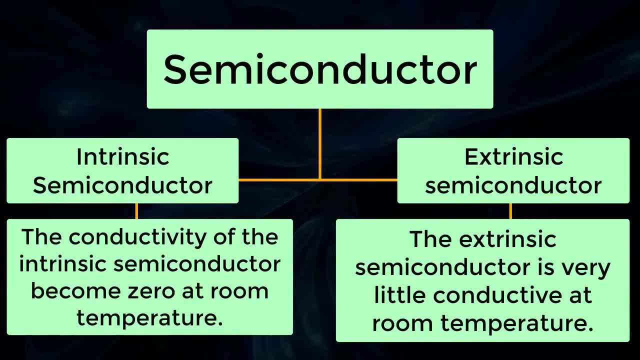 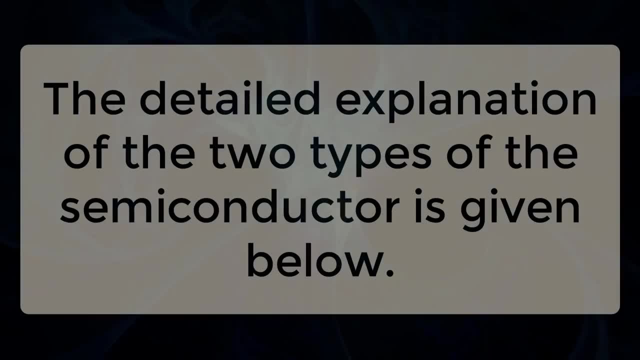 semiconductor. In short, intrinsic is pure, extrinsic is impure. The conductivity of the intrinsic semiconductor becomes zero at room temperature, while the extrinsic semiconductor is very little conductive at room temperature. The detailed explanation of the two types of the semiconductor as follows. 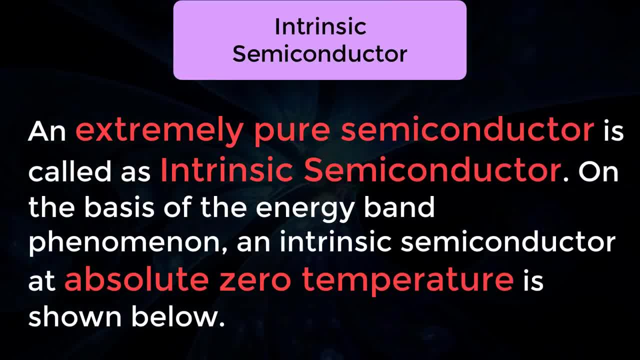 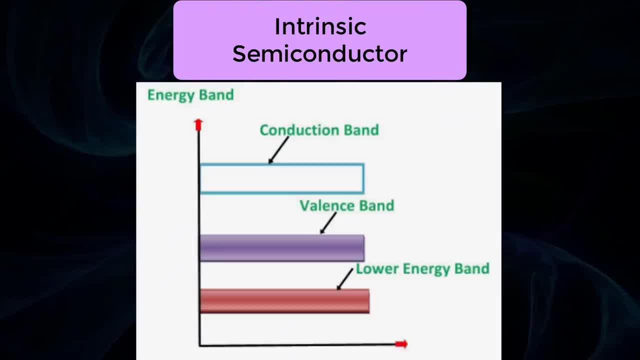 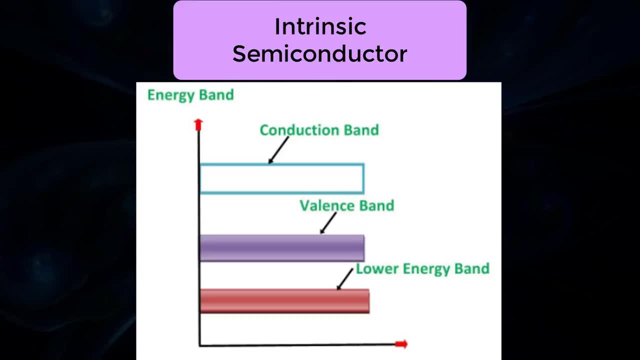 Intrinsic Semiconductor. An extremely pure semiconductor is called as intrinsic semiconductor On the basis of the energy band phenomenon. an intrinsic semiconductor at absolute zero temperature can be seen here. Its valence band is completely filled and the conduction band is completely empty When the temperature is raised and some heat energy. 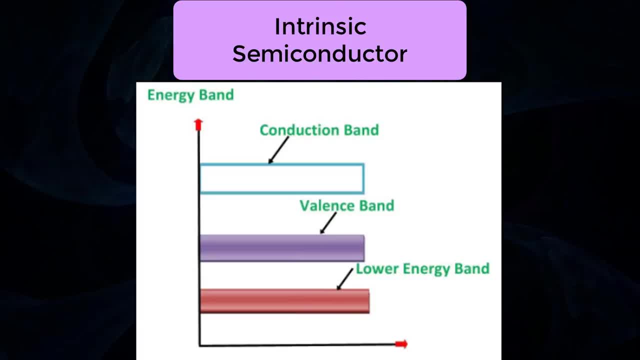 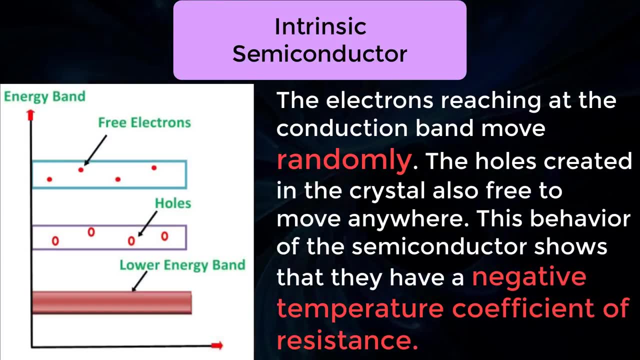 is supplied to it, some of the valence electrons are lifted to conduction band, leaving behind holes in the valence band. The electrons reaching at the conductive band move randomly. The holes created in the crystal are free to move anywhere. This behavior of the semiconductor shows that they have a negative 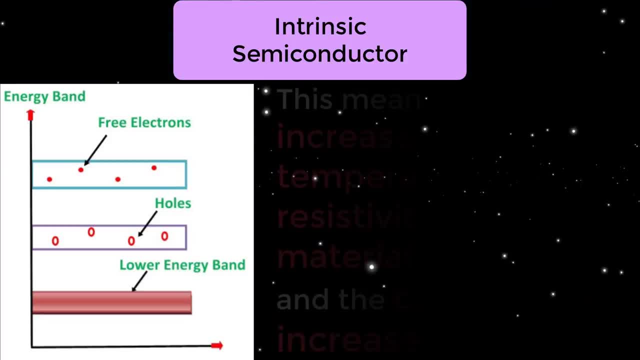 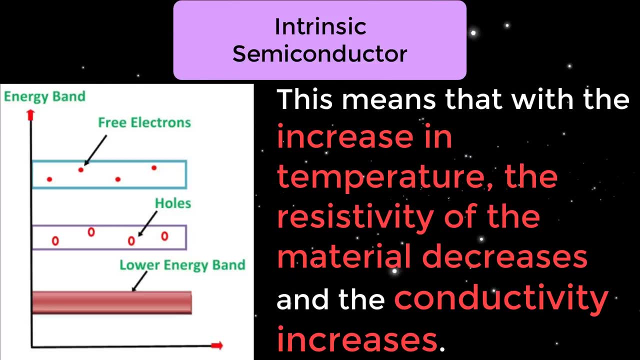 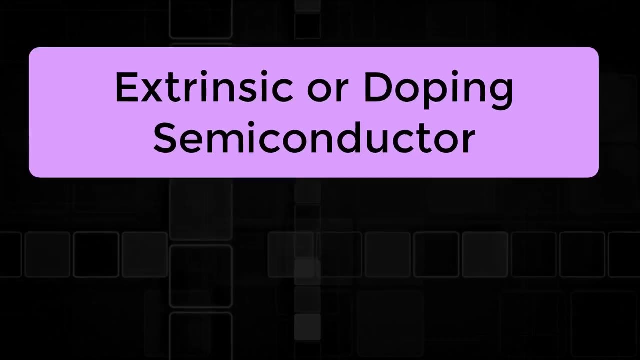 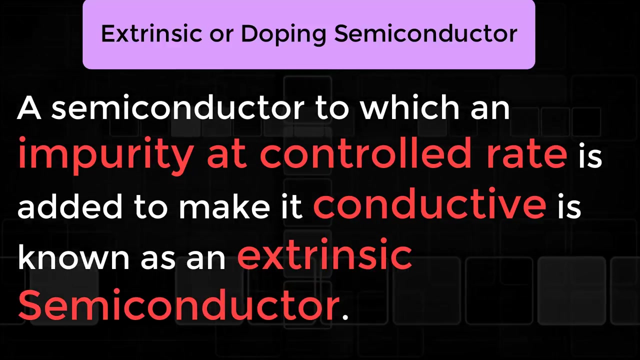 temperature coefficient of resistance. This means that with the increase in temperature the resistivity of the material decreases and the conductivity increases. Extrinsic or Doping Semiconductor. Extrinsic Semiconductor: A semiconductor to which an impurity at controlled rate is added to make it conductive is known. 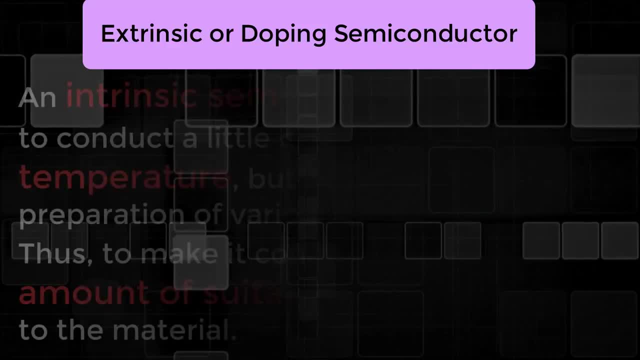 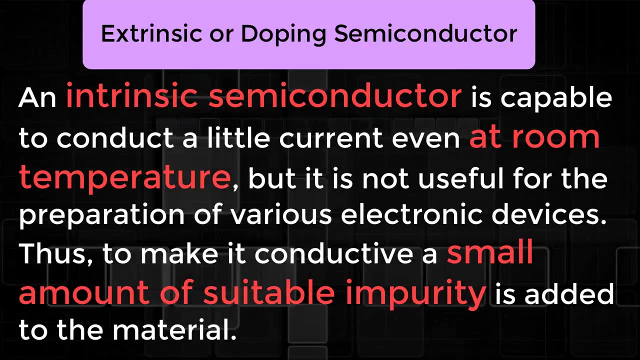 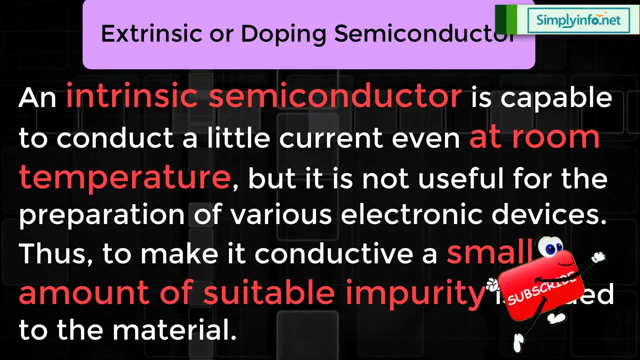 as an Extrinsic Semiconductor. An Intrinsic Semiconductor is capsule is capable to conduct a little current, even at room temperature, but it is not useful for the preparation of various electronic devices. Thus, to make it conductive, a small amount of suitable impurity is added to the material.